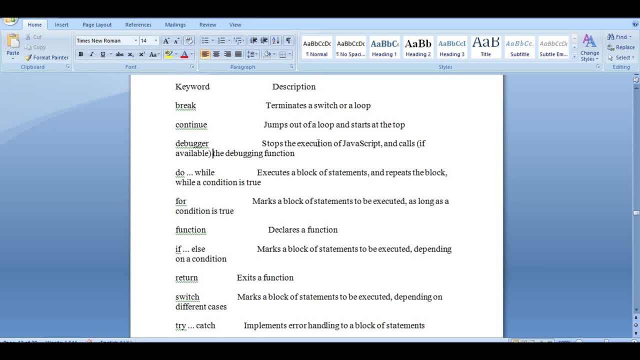 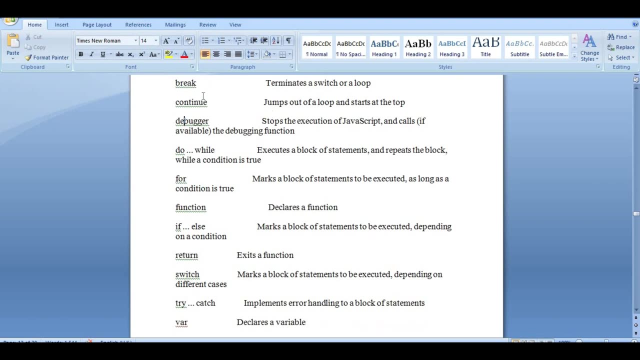 sometimes, if we, if we are making any mistake, it will go to the internet loop and it will not break. in that situation also, you can use a simple break and continue. this continue will jumps out of a loop and starts the starts at the top from where you want to continue. debugger stops the execution of javascript and calls the debugging. 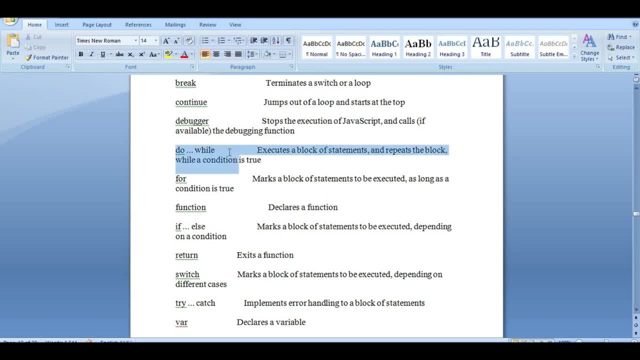 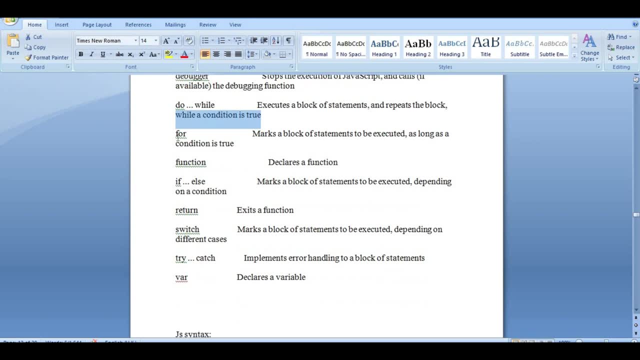 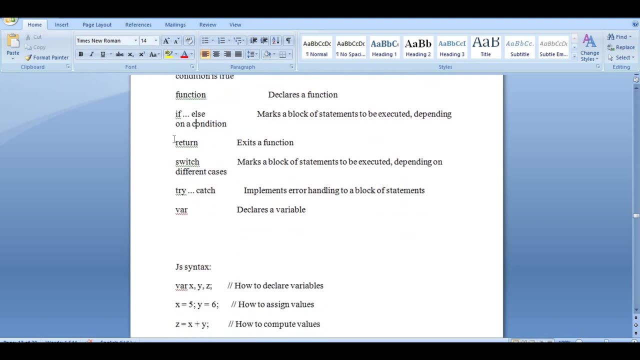 function. so to while is a condition where you can execute block of statements and repeats the block while the condition is true. so all these loops and all we will see in our next sessions, so for this is a for loop function. to declare this function equals: if a nails conditions return to exists a function. 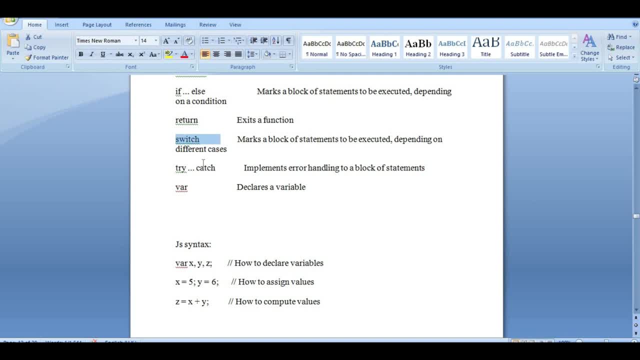 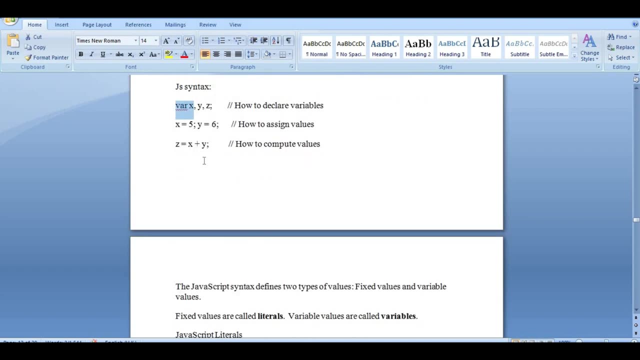 the return values switch. this is the block. block statements: right catch, if you are any. if you are having any error, you will catch that error. this var declares a variable. just now we have seen, so here i have shown you var: x, comma, y comma, z, then x equal to pi and y equal to six. 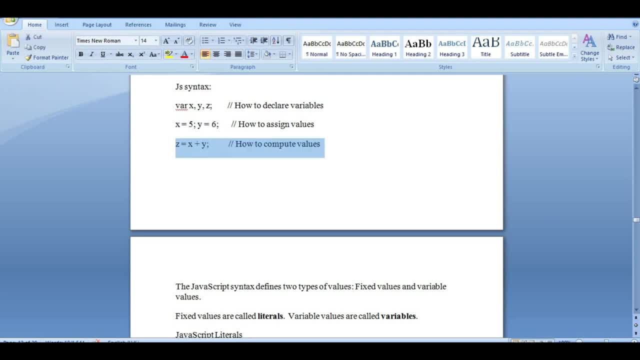 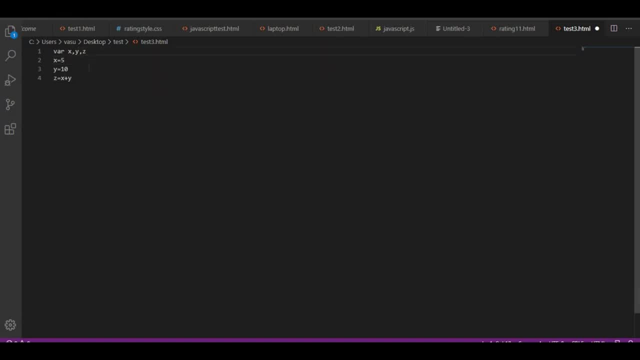 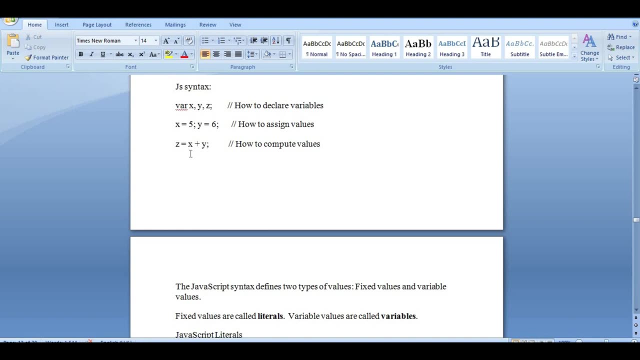 will assign the values and this is how we will compute the values. sorry, i did not give here z typing here. i have used z, but if you are doing any program you will get the error. if you are not ready, so in the, in the, in that cases you can correct it. so this is how you can compute the. 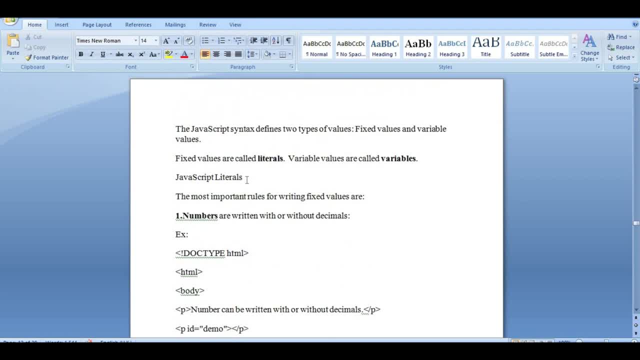 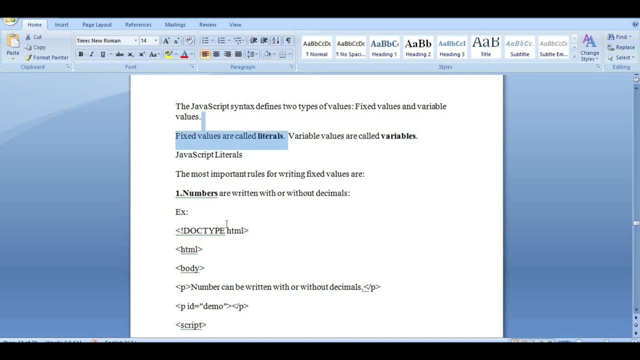 values that equal to x plus y. let's come into weight values. you will have two values: literals and variables. so what you call as a literal is the. if the value is fixed, then it will be called as literals. if the value is changing, that means if the value. 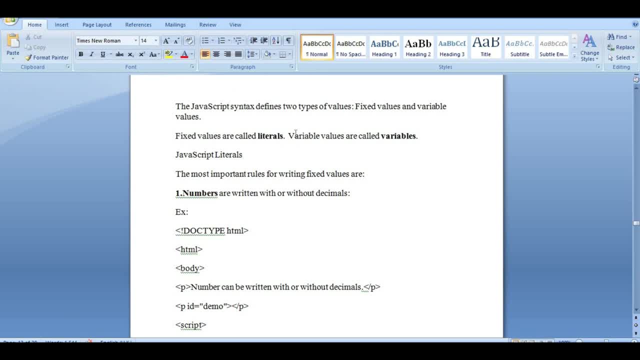 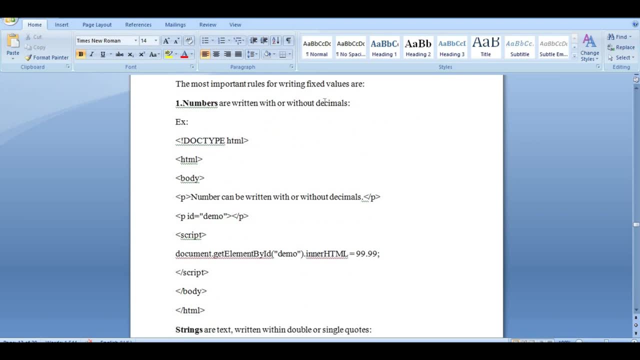 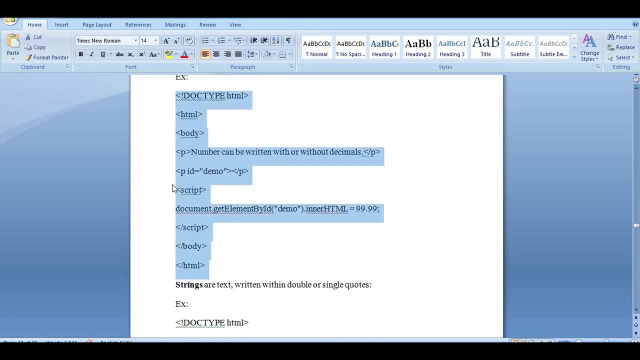 is uh, keep on changing. then it is called as variables. then from then coming to the rules. first rule is: numbers are written with or without decimals. we can use either the decimal or we can without the decimal. so you can use. i have written a simple program. i will show you. 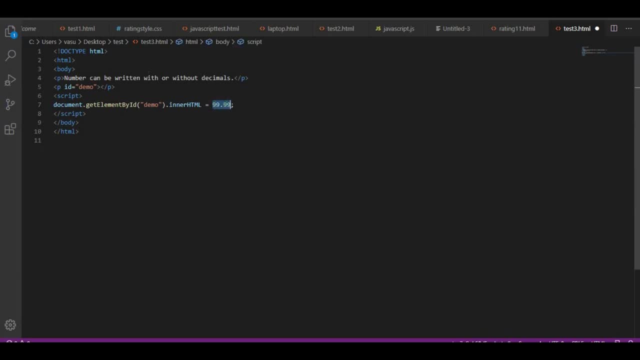 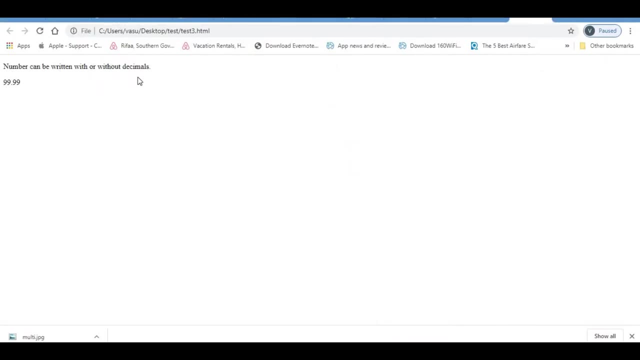 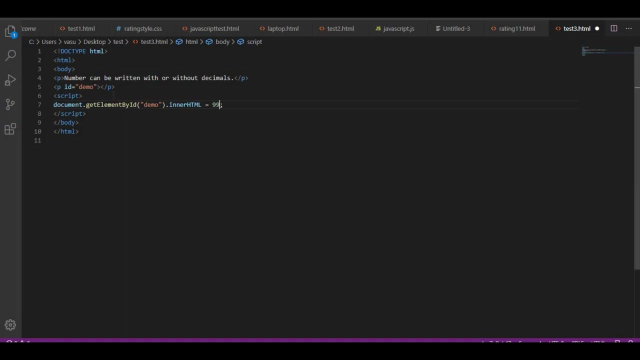 here i have written the number with decimals, 99.99. so let me try to execute this. see, numbers can be written with or without. 99.99 is the number. so next, i will not give decimals. that means it can be acceptable with note or any types of numbers. 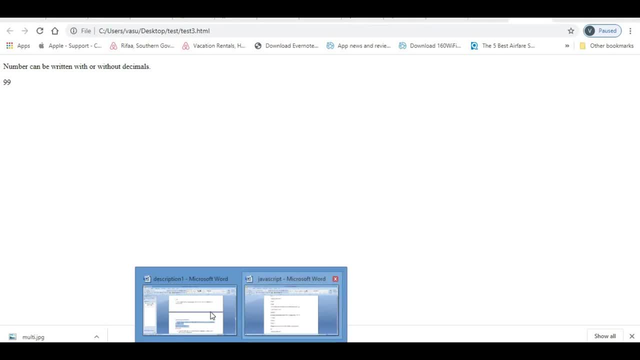 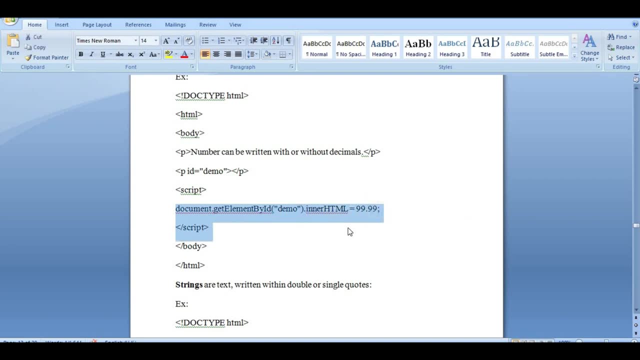 so 99? i've got it as 99. so this is how you can give the numbers. so here just i have given document or get element by id. you know, in the html i have used for this explanation i have already told you in my previous sessions- you can see that 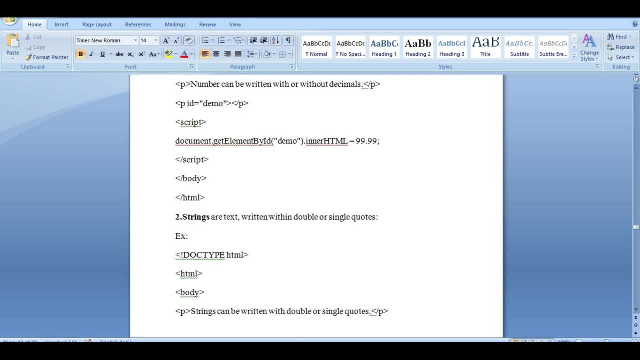 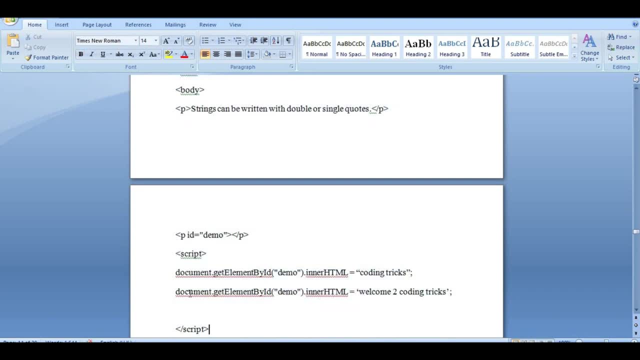 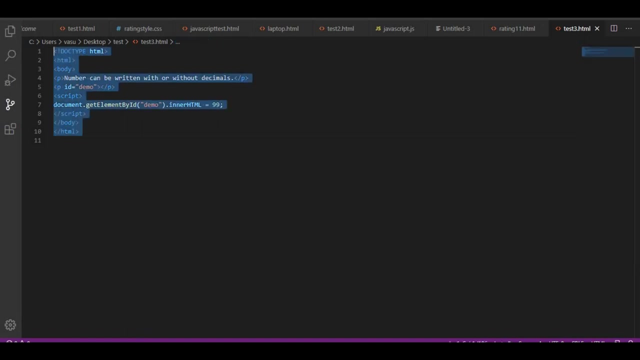 so next one, next syntax is. second one is strings. so strings can be used with a single code or with double codes. so we can use a single code string or we can also use a double code string. so you can see a simple example. now i'll show you something else. for example, here you can see the document would get element by id. 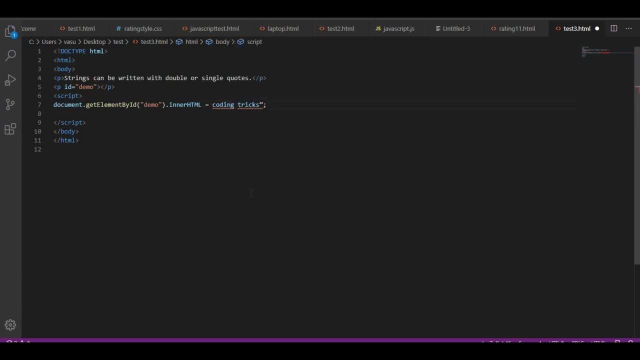 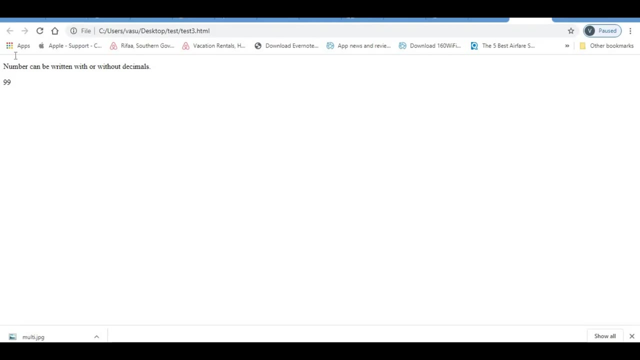 inner html coding tricks. here i have used two double. here i have used double codes, so it will print one quad s. then we see here coding tips: strings can be written with double codes or single codes. so now i will give the single codes. so this is what i have written with single codes. 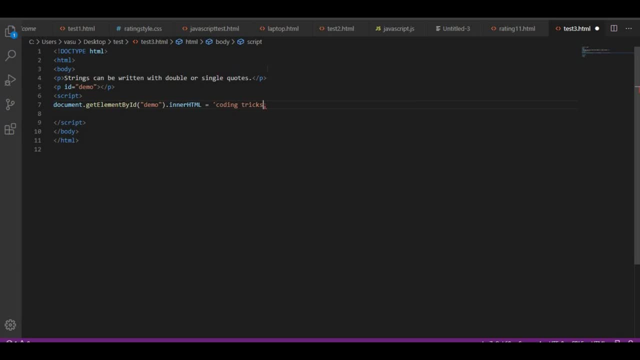 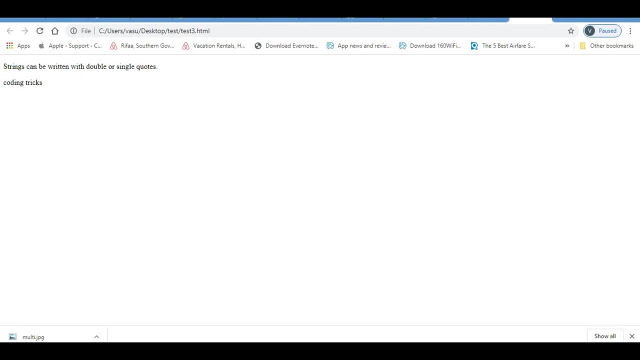 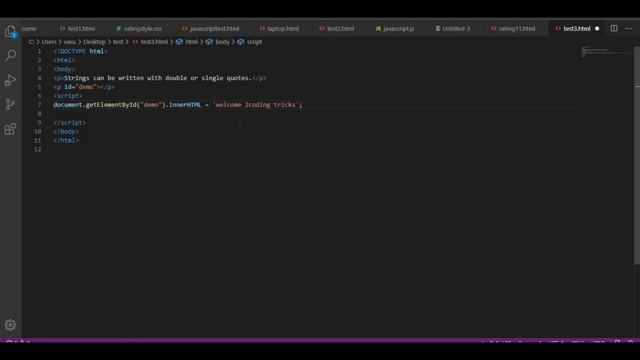 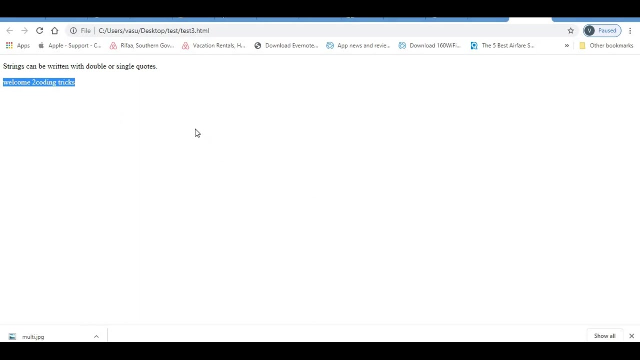 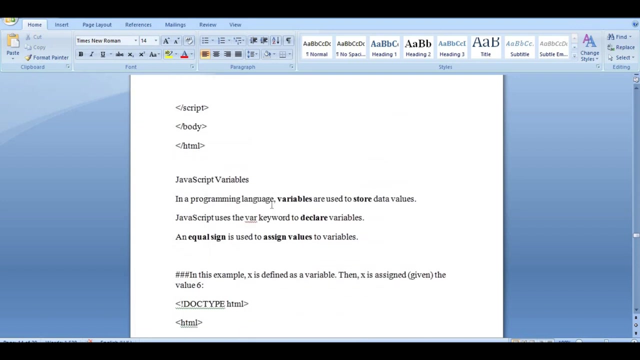 So this is how you can write a string with single codes or the double codes. Next is JavaScript variables. So in programming languages, variables are used to store data values. So here I have used the variables x, y, z. Why I am using 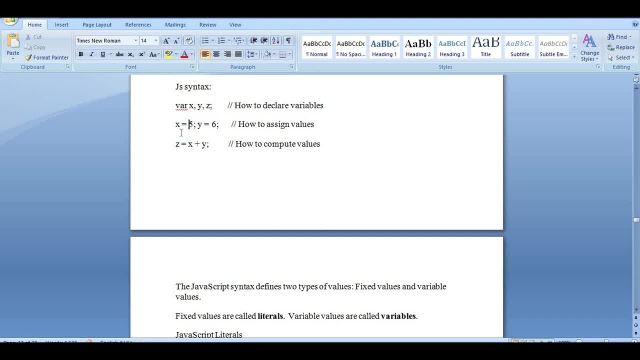 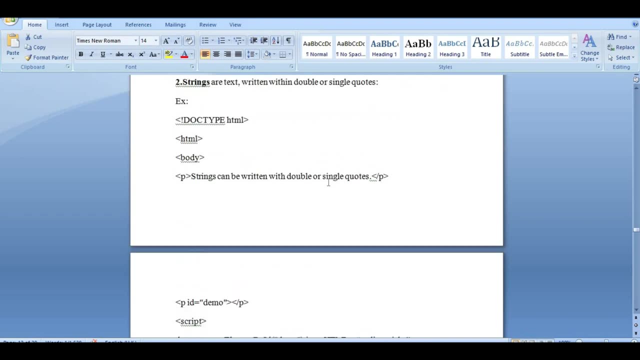 To store these values x equal to 5.. In order to store this value 5, I am using this x variable. So here I have used 6 and here I am adding up and it is storing in the variable called z. So, in order to store the variables, 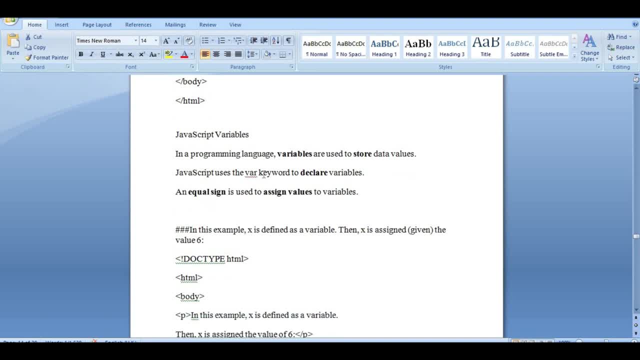 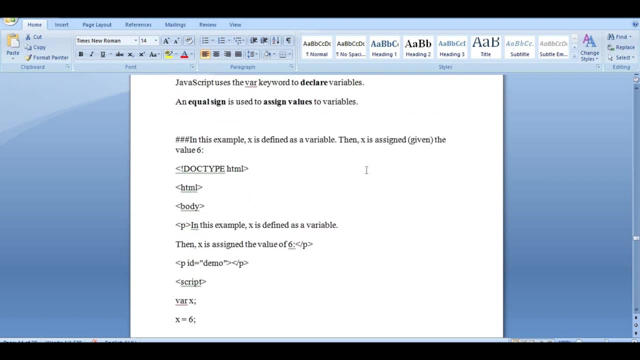 we will use variables. So JavaScript uses the var keyword to declare variables And equals sign is used to assign the values. All these we have already shown, So I will show you one more example. Here x is defined as a variable and is assigned the given value. 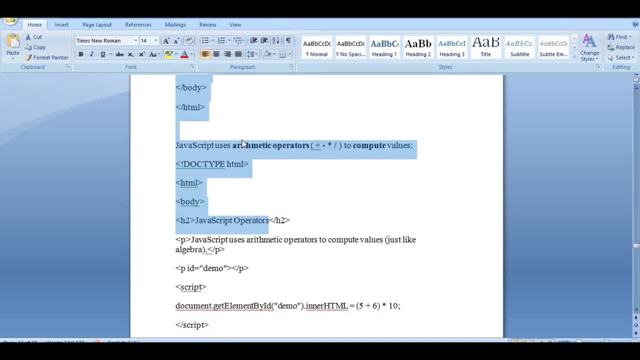 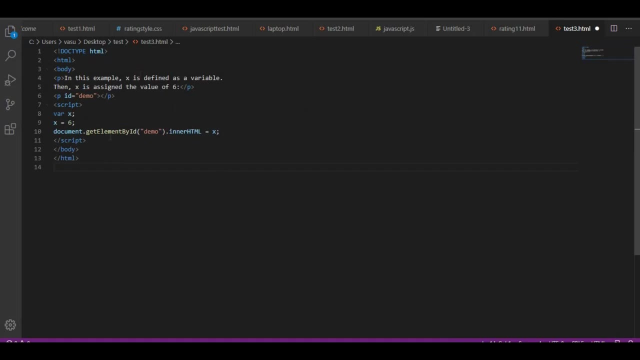 So let me show you this example and I will explain you. So I am going to paste this. So what I am doing here is in this example, here x is defined as a variable, Then x is assigned the value of 6.. So here now we have seen where x, y, z we have declared in the previous class. 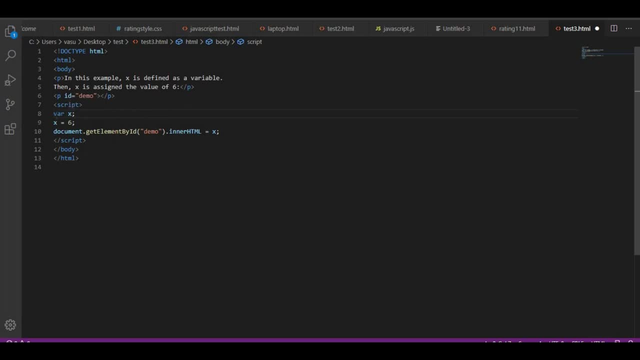 in the previous just now. So where x, x equal to 6. And here I am asking: yes, So let us see What is the output you will get as 6.. This is how you can use So document: dot. get element: my id: demo inner html. 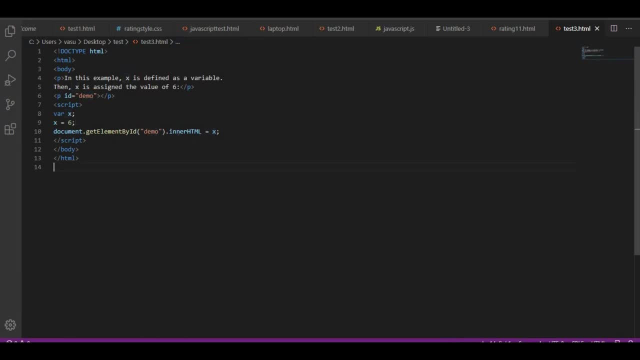 So, about this demo and all we have already seen, because since we have using here demo and I am using and I am calling here like I am using the same name- identifier name, So I will get the value of x Here, Okay. So next, 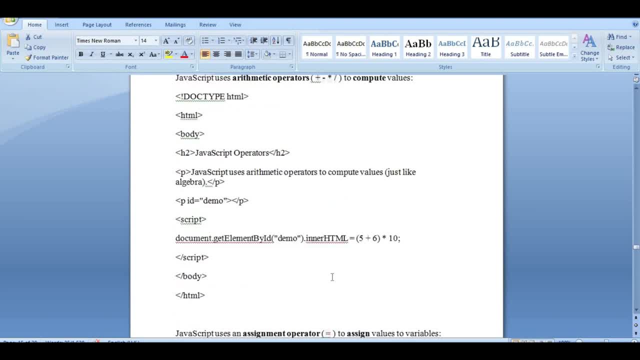 Arithmetic operators. So we can also use the arithmetic operators or any operators with this. So here I am using document dot. get element my id, demo 5 plus 6 into 10.. Then you will get. it will be solved by bracket plus, then multiplication. 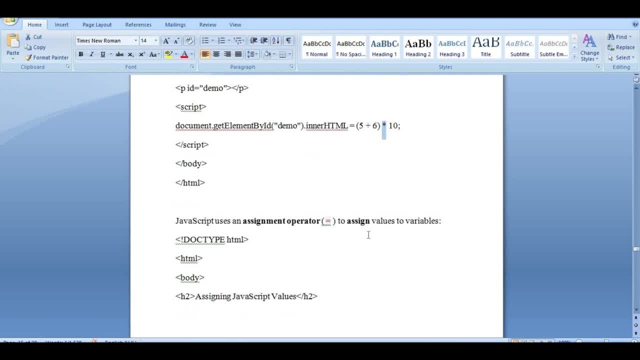 So you will get 11 into 10 is 110 you will get For the operators and all I will provide you in detail class, in detail session, So you can see to that. So this assignment operator will assign the values As if, like where x, comma, y, here I am assigning the value of 5 to x. 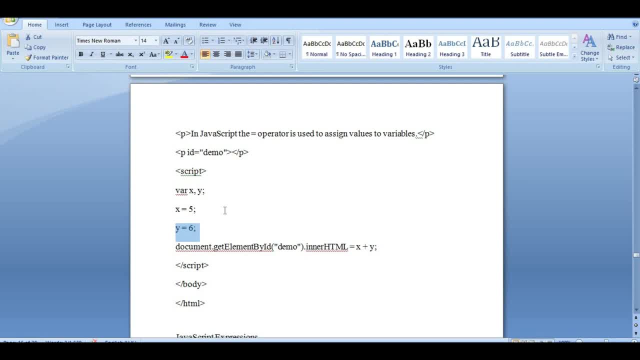 y equal to 6.. So I am assigning the values over here. So 5 is x is assigned with 5 and y is assigned with 6.. It will store the values over here. Javascript expressions, So an expression. we know that expression is a combination of values, variables and operators. 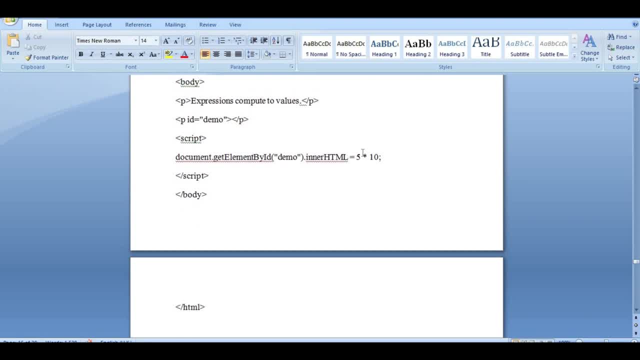 Which can compute the values. So here we are using the operator and values, So it will compute the value and it will give you as the result: Expression can also contain variable values. Yeah, This is a good example. I will show you. 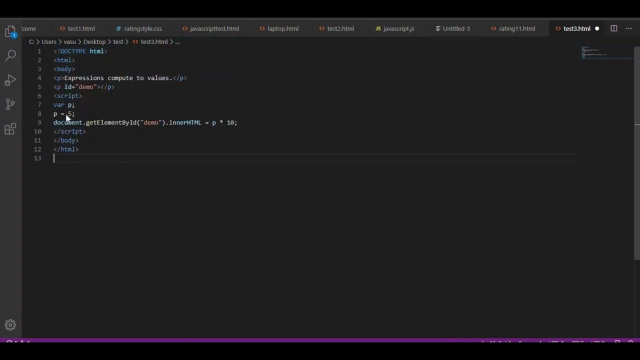 So here I have used the value p, So I have initialized p with 5. And I am calling sorry and I am using p into 10 here, So I will get 5. 5 into 10. I should get like 50, I should get. 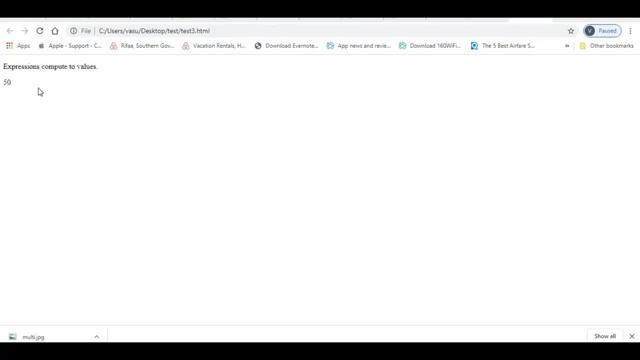 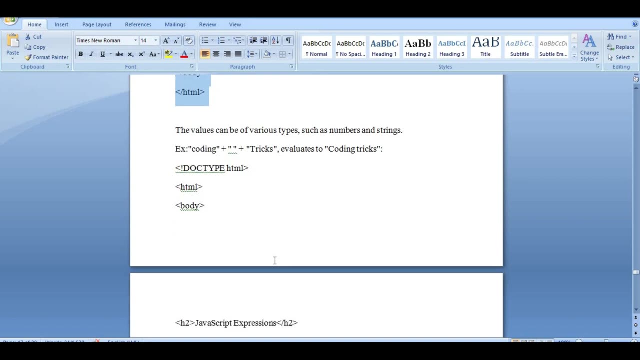 So let me see: Yes, Expression compute values is 50.. This is how You can assign the values. Next is the values can be of various types, such as numbers and strings. So here, Yeah, This is also a good example. 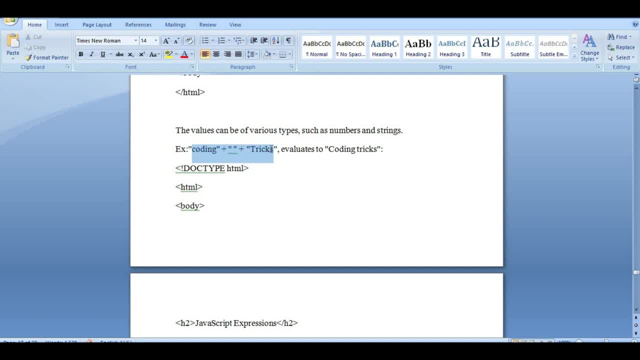 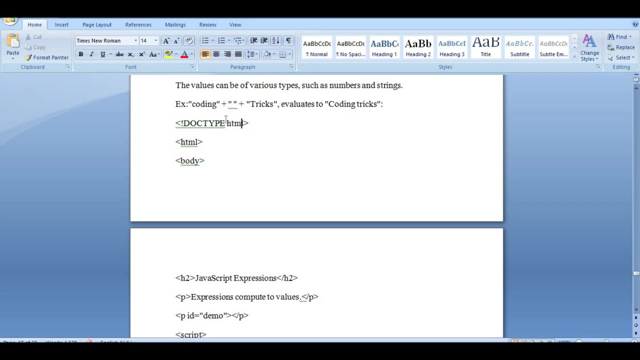 Here I am using coding and tricks. So if I want to concatenate, If I want to combine these strings, I will use plus operator here. But if two strings can be concatenated with the help of plus, Two numbers can be concatenated, Two numbers can be added together with the help of plus. 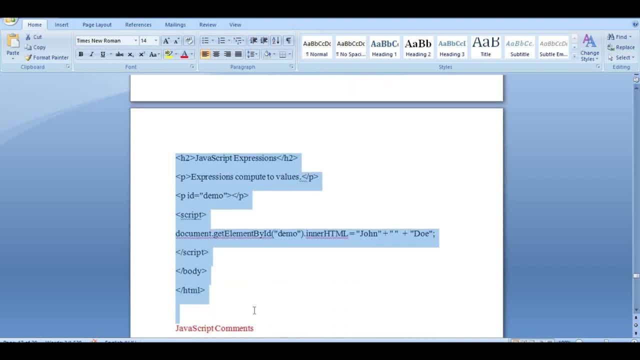 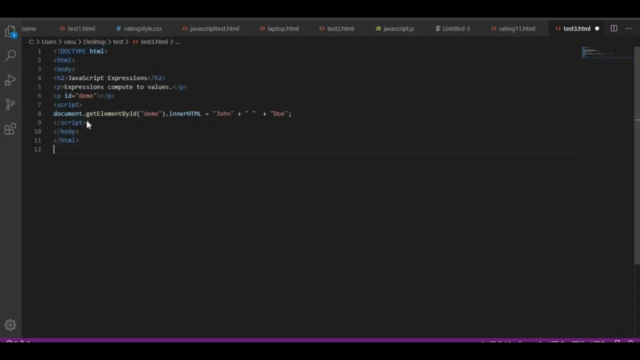 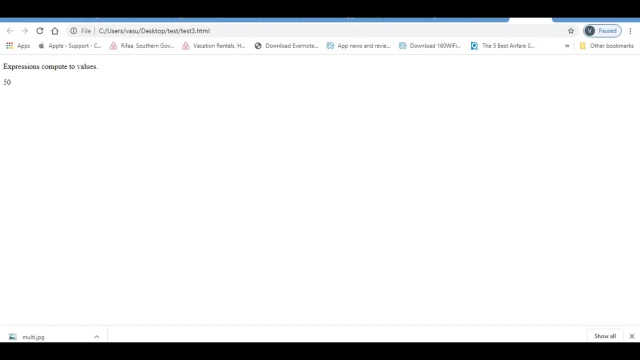 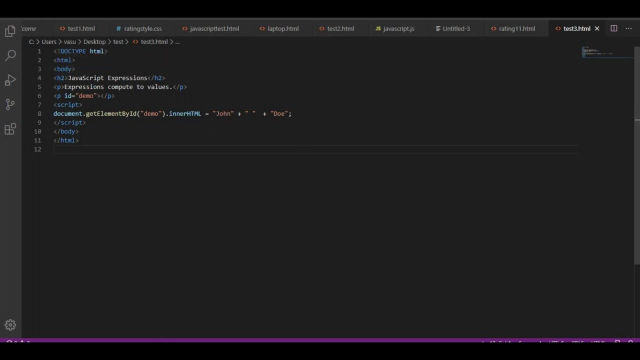 Here I am using for concatenation. That means two strings should be combined together. So here I am using two strings, Like: Yeah, Here I am using John and Lloyd. So let me try this: John and Lloyd, Oh my god. 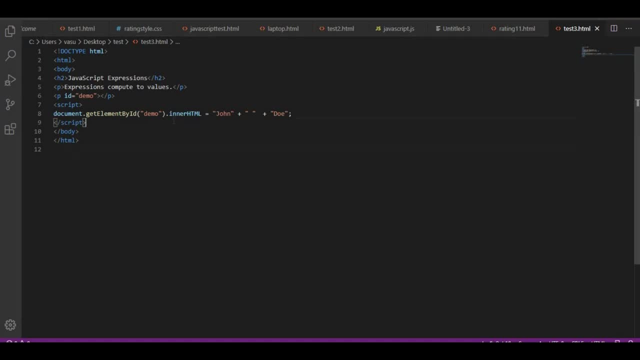 That means what I want to tell you here is: So here I have used plus operator. So why I am using this is To get the space in between these two, So here you can observe the space over here, right. Without that you will not get the space. 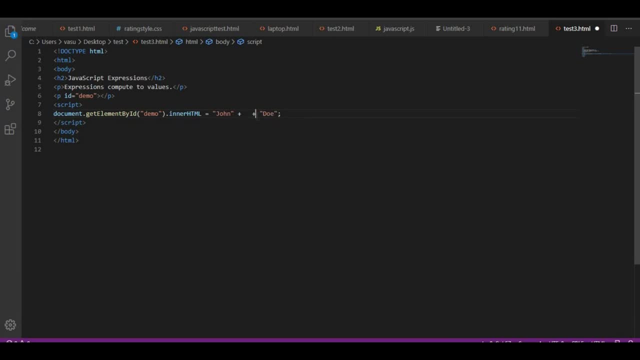 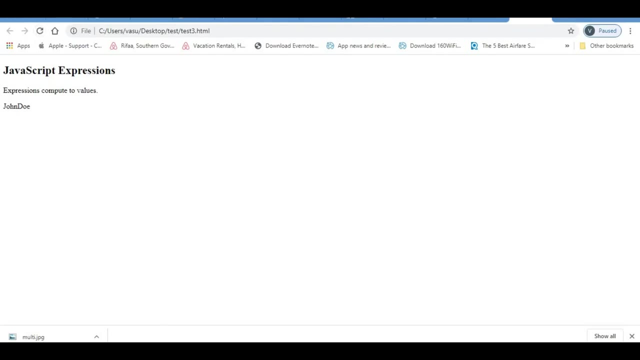 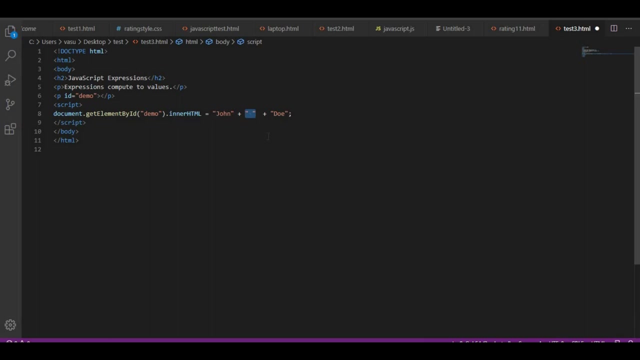 So let me remove that. You will see, You will not get the Space. So this is how. So why I am using that plus with the parentheses To get the space. If you want to get the space You want to use. 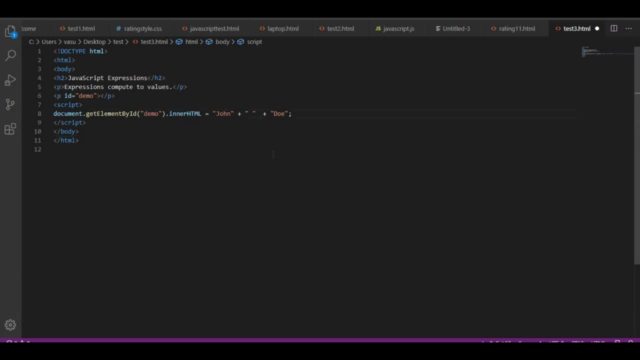 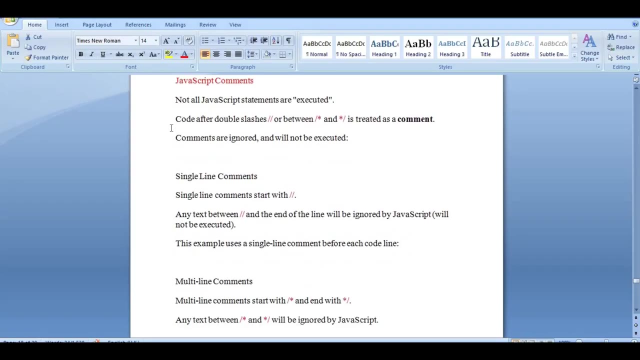 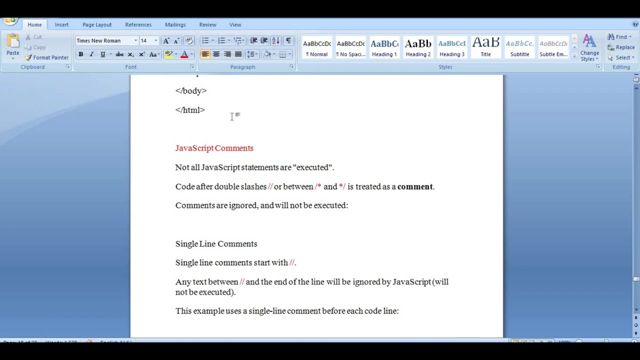 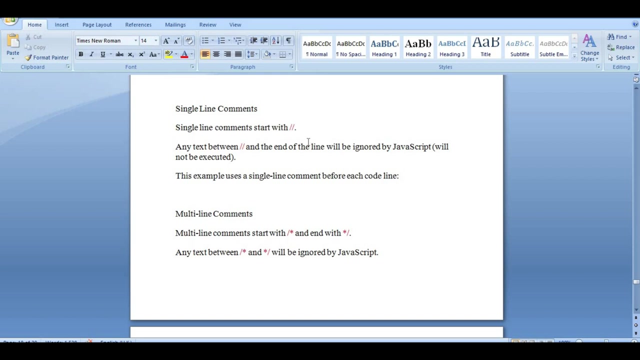 This Plus and inverted commas, Double quotes, Then javascript comments. So javascript comments can be done with single line comments and double line comments. So these javascript comments cannot be executed. That means it will not be executed Any Any Any statements cannot be executed. 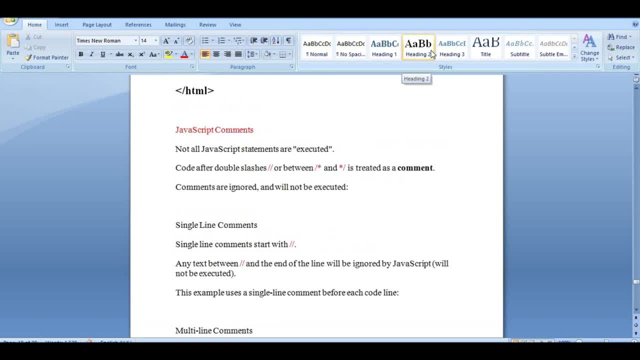 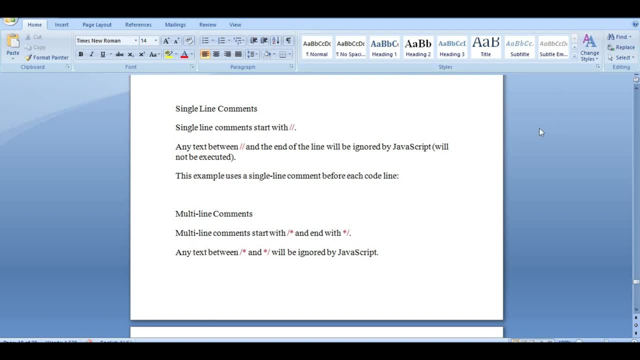 So if you are writing in a commas, Why we are writing commas is If A programmer, If you are writing a program and giving to the other person, The other person should also Be able to understand your program. So That's why we are writing the commas. 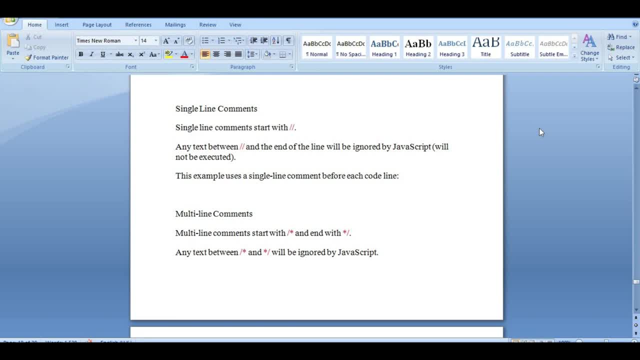 For example, I am, I am declaring the values: If: 1. Where x equal to Where x, my z and x equal to 5.. y equal to z, y equal to 9., Then I will write a comment. 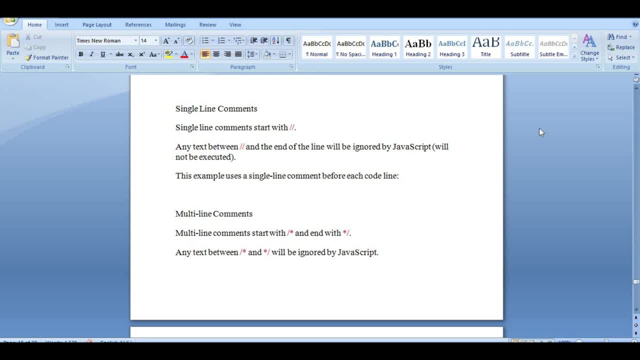 Here I am going to perform addition z equal to x plus 5. Then the other developer can understand that he is doing the addition. So in that situation these comments are used. So now let us see a simple example for single line comment. 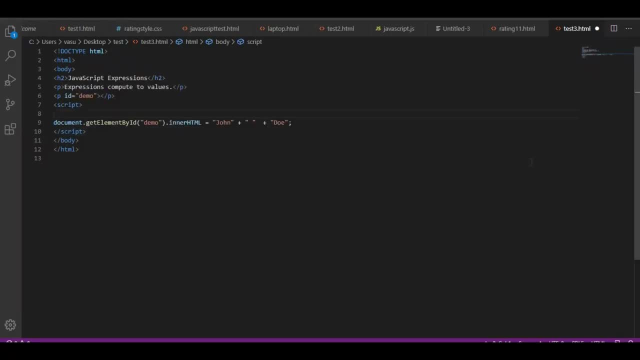 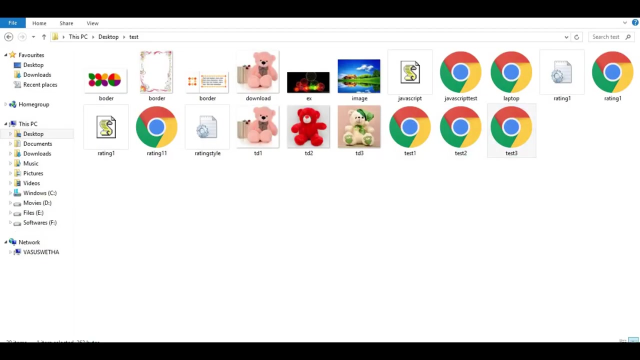 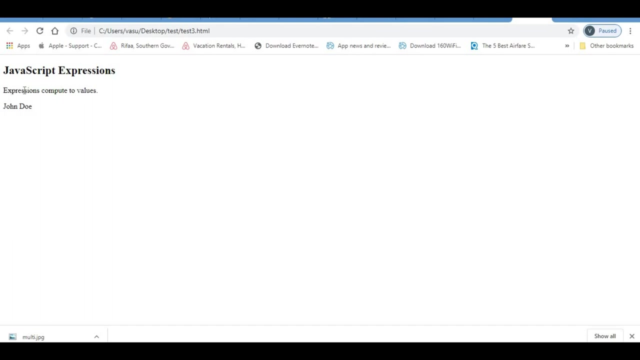 So I am going to write Simple line comment here. Here will write concatenation, because i am concatenating two strings, concatenation of two strings. so i'm going to write this, so i'm saving this, then i'm trying to execute: yes, so see here, you did not get the one comment: concatenation of two strings. 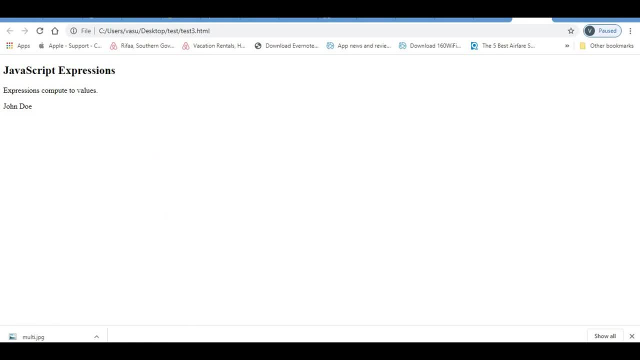 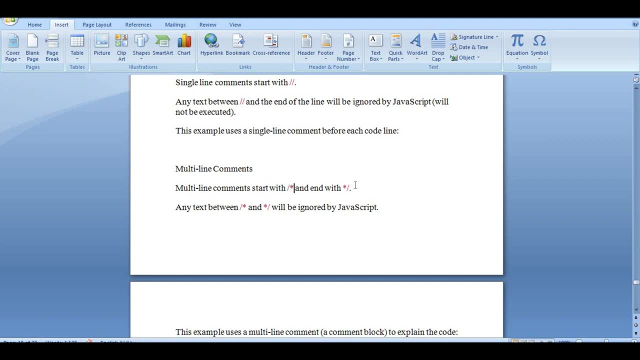 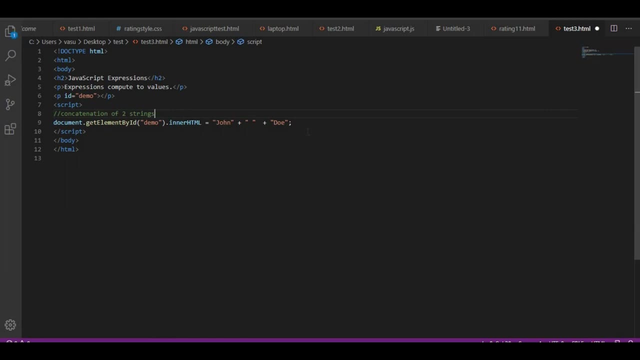 so that is how you will give the single line comment. coming to the multiple multi-line comments, you will go with this: slash, asterisk, asterisk and slash. so if you are having multiple lines comments, so then you will go with this. for example, i will go with this: